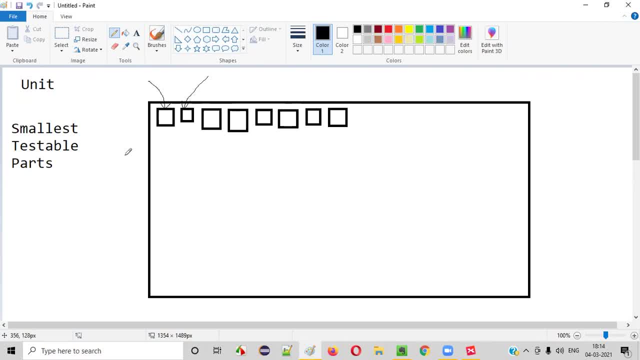 this unit you can test individually this particular smallest testable part. that is unit. you can test individually, like that if you want to. if you are testing each and every smallest testable part, that is unit individually. this thing is known as okay. this type of testing is known as unit testing. it is one of the levels of software testing where you are testing the. 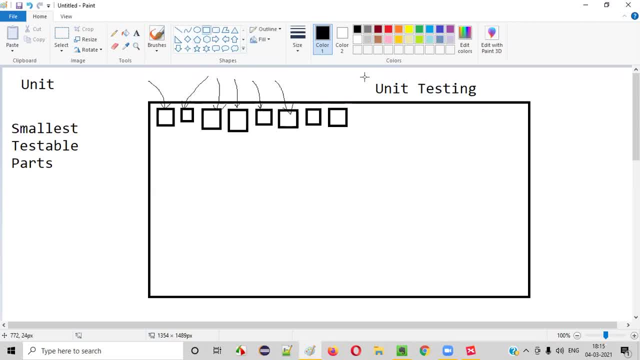 smallest testable parts, that is, units. nothing but unit testing. fine, now let me explain more about this unit testing. okay, so what exactly the units are. if i have to programmatically represent a particular unit, it will look something like that: guys, i will take the example of the java guys- i want to represent a unit in terms of java language. i'll create a. 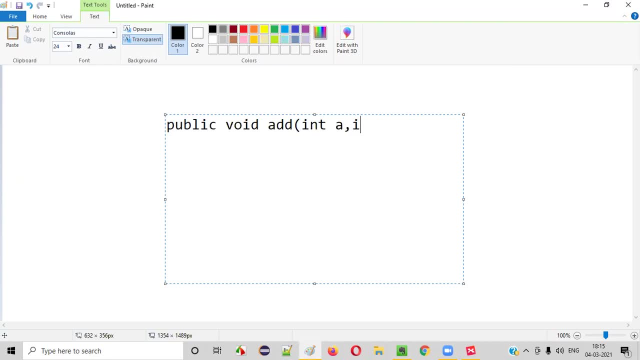 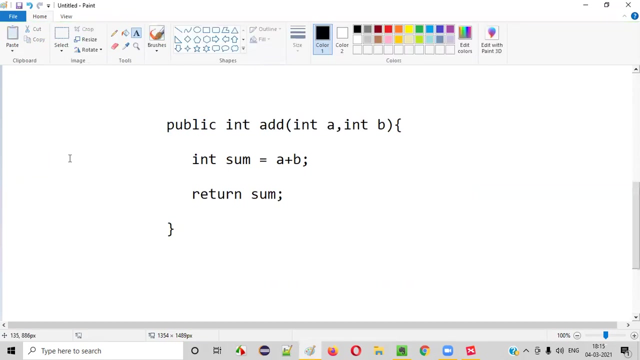 method like this: public void: add int a comma, int b. okay, this is a java code, guys, so this code cannot be broken further. okay, this code cannot be. i'll say something like this: int sum is equal to a plus b. and then here i will say return sum. here the return type is int. let's say so. this is a sample. 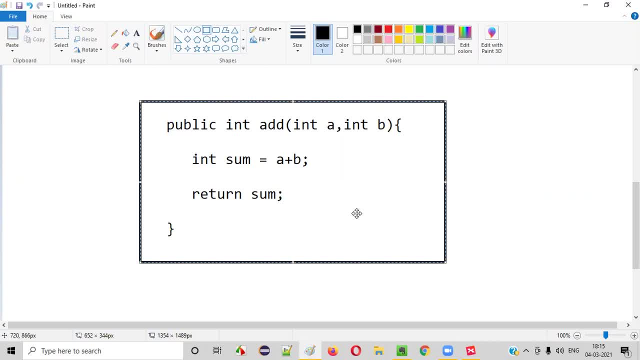 code for a unit. guys, you cannot break this unit further. okay, this is smallest testable part you can say, which is nothing but a unit. how to test this particular unit individually or independently? how to test this part, the parts, particular unit, guys. so here in order to test this particular, smallest testable part, that is unit. 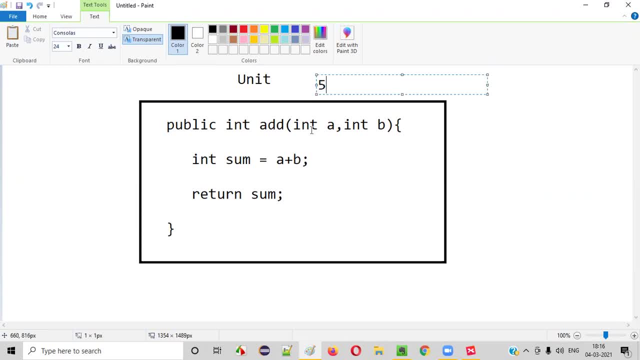 what we'll do is we'll pass two values. let's say i'll pass 5 into a and 6 into b. what is the result, guys? 11. this is one test. similarly you can pass. you can do another test. say here you will pass 8. 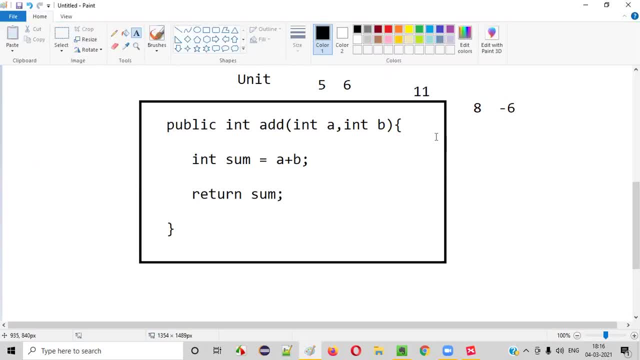 and here you will pass minus 6. 8 is passed to a, minus 6 is passed to b and if you are getting the result, okay, the return. if this particular code is returning you something like 2, then this test is successful. so here we are performing unit testing like this, guys, we are testing the.